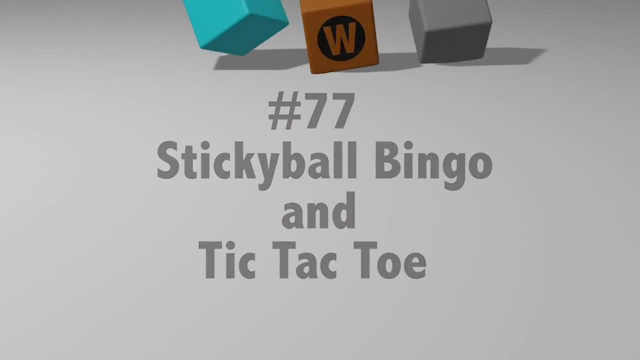 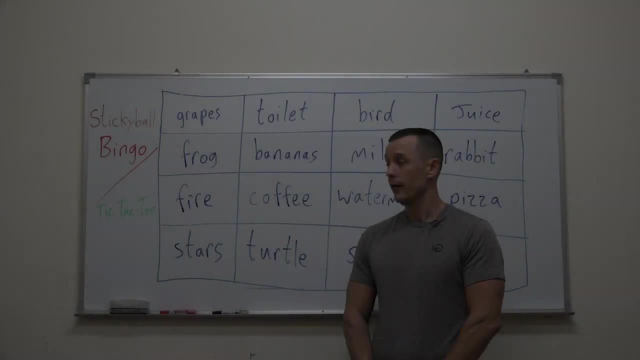 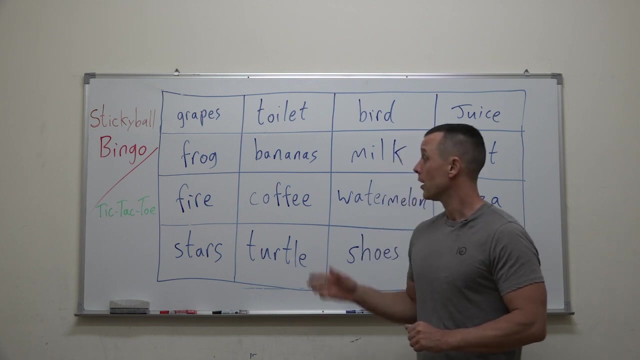 Hi everybody. this is Dustin from Guys with Games. Today's game is called Sticky Ball Bingo, or you could play the Sticky Ball Tic-Tac-Toe version, Okay, so right here, this is the Sticky Ball Bingo version, and I have a 4x4 grid, so I have 16 words on the grid, Okay, 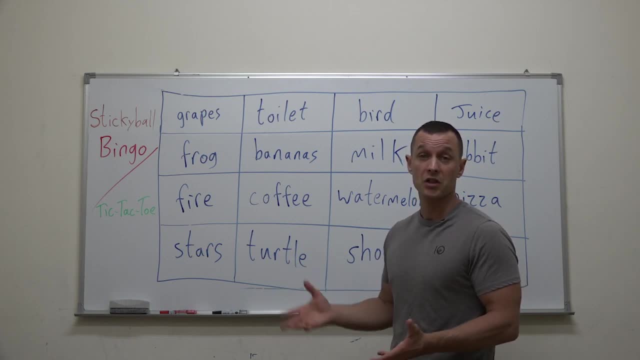 you could also have a 5x5 grid if you want to and have 25 words. it'll just take longer. if you have more students, you could do that. So what I'll first do if I'm reviewing these words with the kids, I'll say: grapes. what are grapes? Is it an animal? And they're like. 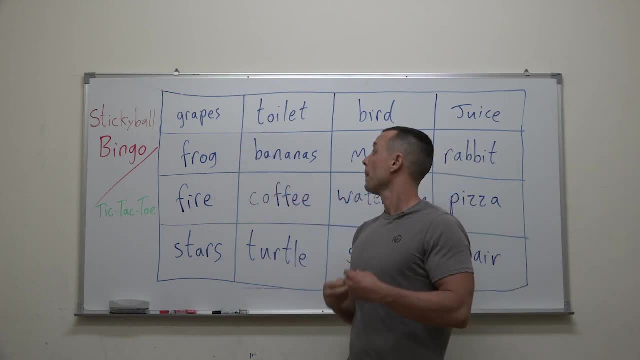 no, I'm like, what is it? And they're like a fruit Good. Are they big or small? Small And I'll ask. I'll try to elicit answers from the kids, try to get them to describe these. 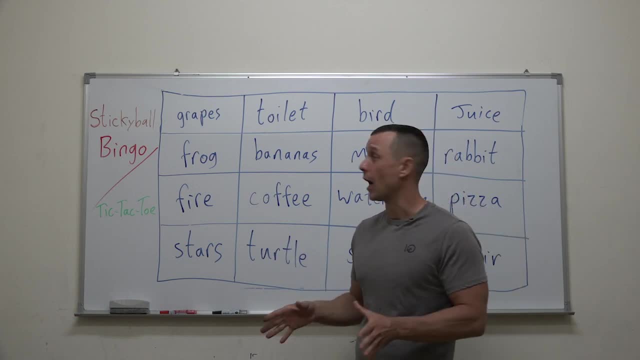 words. Okay. so depending on how much time I have will depend on how much time I will go through each of those words. Okay, so I make sure that the word that they know I don't put in a new word, Vocab up here. I'm going to pair off the students, So I'm going to divide the class into two. 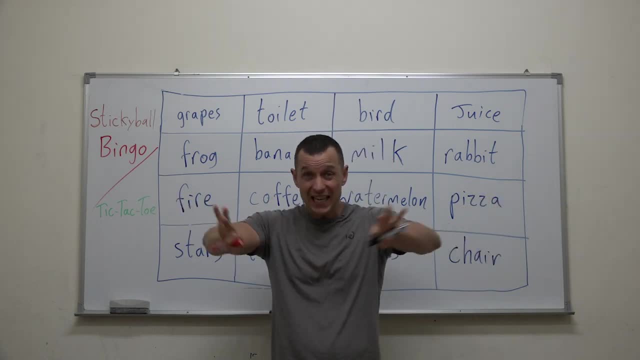 teams, team A and team B. For each team I'm going to assign number one, number one. So there's two number ones, one on each team: Number two, number two, number three, number three, number four, number four, number five, number five, number six, number six, So that's. 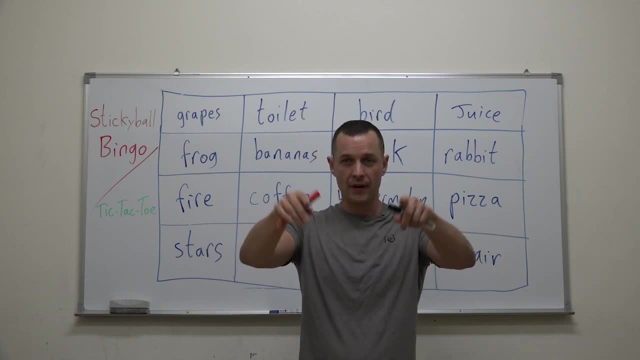 if I had 12 students, So 1, 1,, 2,, 2,, 3,, 3,, 4,, 4,, 5,, 5,, 6,, 6.. Okay, And so then what I? 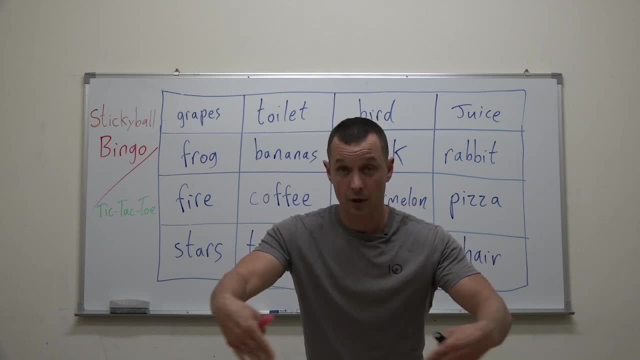 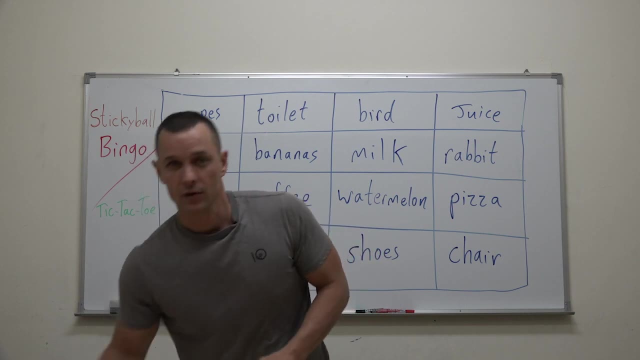 do is I draw a line on the floor, Or you make a mark on the floor, or you just have a line where the kids are going to throw from from the floor. I put this: stick, two sticky balls there, Boom, And then I will. 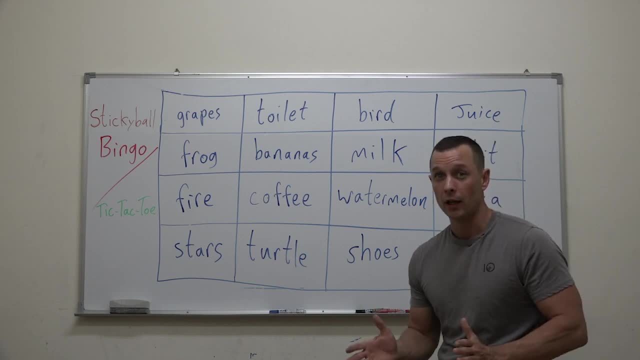 describe a word, I will say it's a drink, But as you can see, there's more than one drink here. I'll be saying it's a drink, It's white, It comes from an animal, Number four- And then number fours will have to come up, and they will have to. whoever hits milk first is the winner.